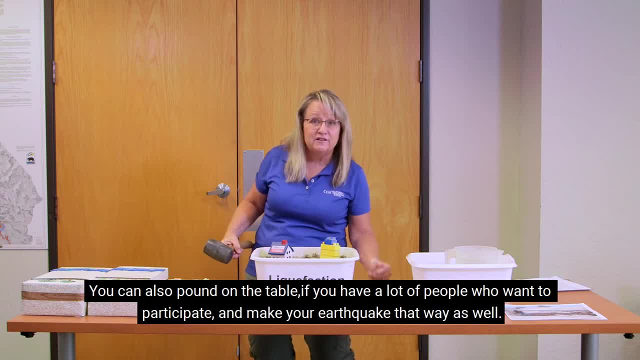 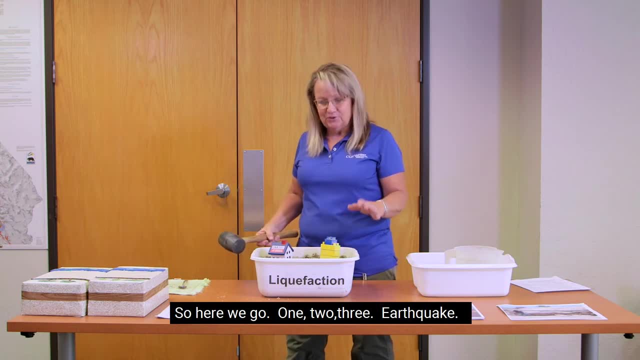 I'm just going to tap on it and get it vibrating. You can also pound on the table if you have a lot of people who want to participate, and make your earthquake that way as well. So here we go: One, two, three Earthquake. You watch the surface and you can see what's happening. You can see. 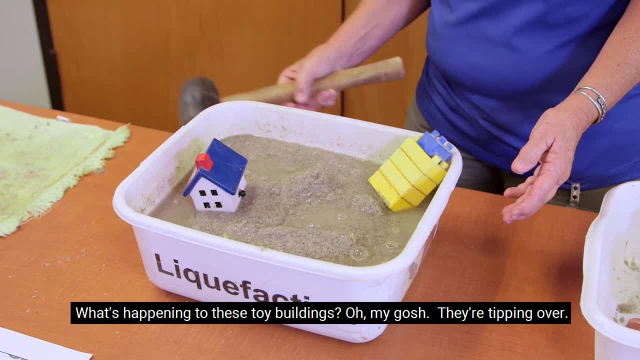 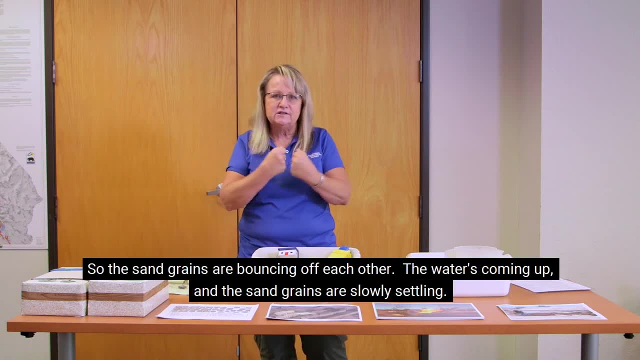 the water's coming up. What's happening to these toy buildings? Oh my gosh, they're tipping over. What's happening to the pipes? The pipes are coming to the surface, just as we predicted, So the sand grains are bouncing off each other. The water's coming up and the sand grains are. 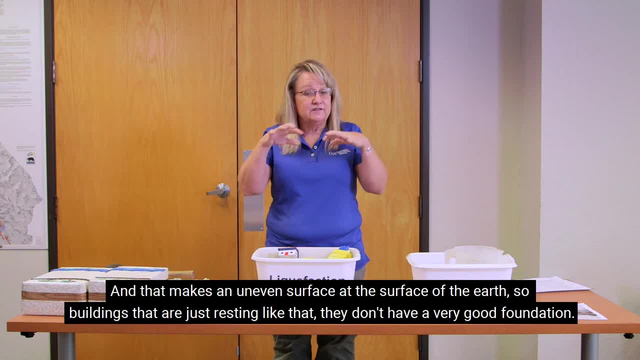 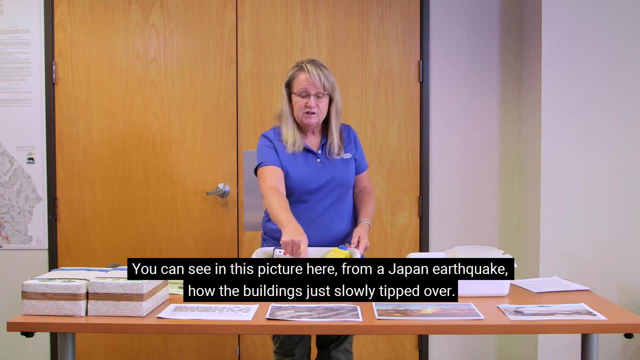 slowly settling and that makes an uneven surface at the surface of the earth. So buildings that are just resting like that they don't have a very good foundation. You can see in this picture here from a Japan earthquake how the buildings just slowly tipped over In that earthquake. no one 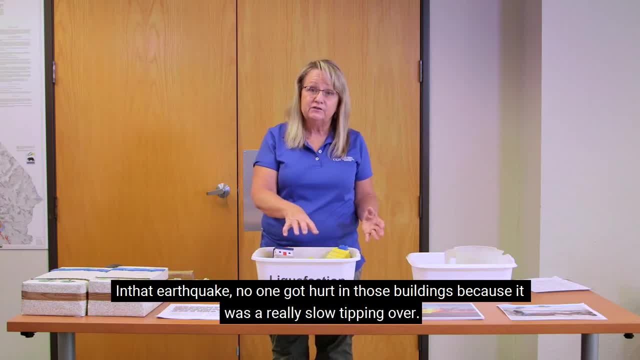 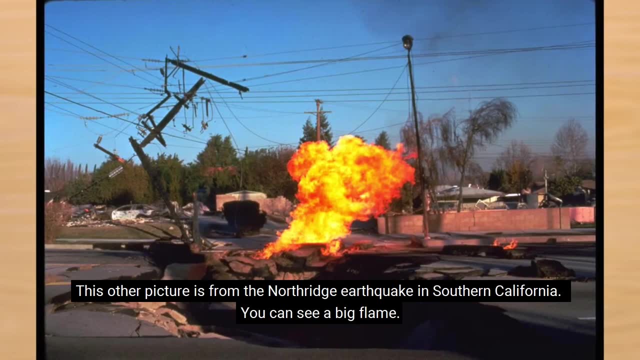 got hurt in those buildings because it was a really slow tipping over. But after that earthquake we learned more about how to make buildings safer in areas where liquefaction can occur. This other picture is from the Northridge earthquake in Southern California. You can see a big flame fires coming out of the street there. 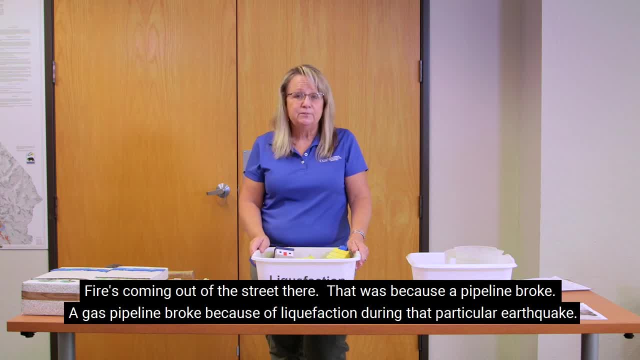 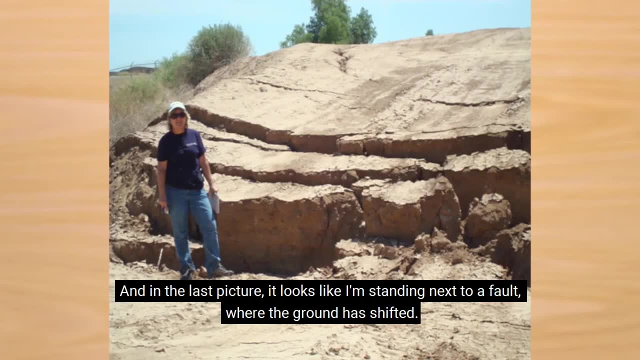 That was because a pipeline broke. a gas pipeline broke because of liquefaction during that particular earthquake, And in the last picture it looks like I'm standing next to a fault where the ground has shifted, but what happened is that's actually settlement due to liquefaction. 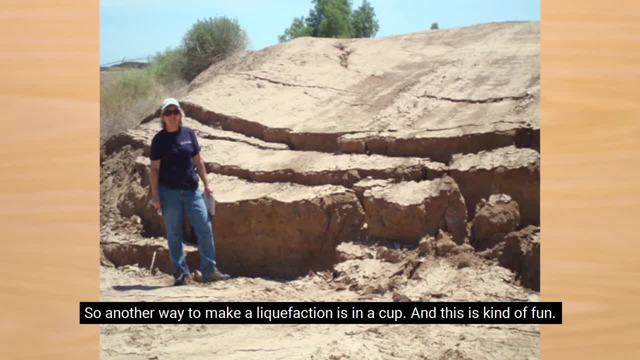 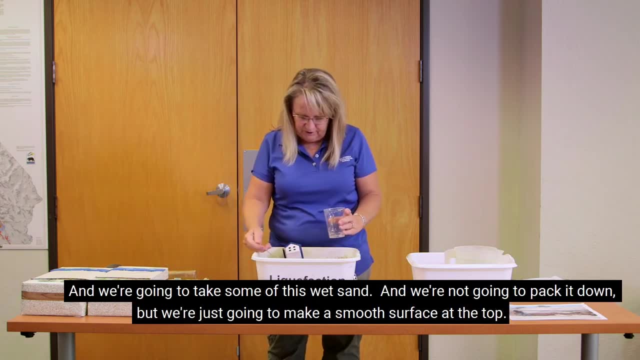 that occurred in an area down in Southern California. So another way to make a liquefaction is in a cup, and this is kind of fun. If you have a classroom you can let everybody be doing it, participating with their own cup. But we're going to take some of this wet sand. 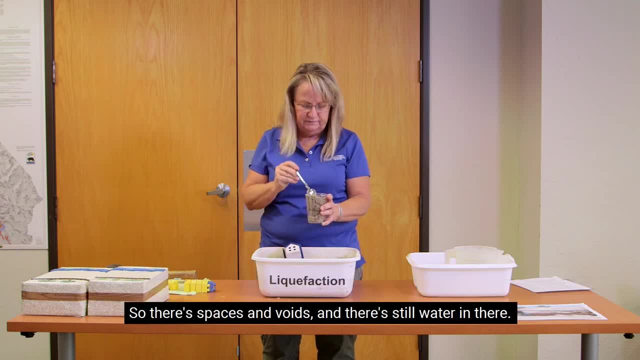 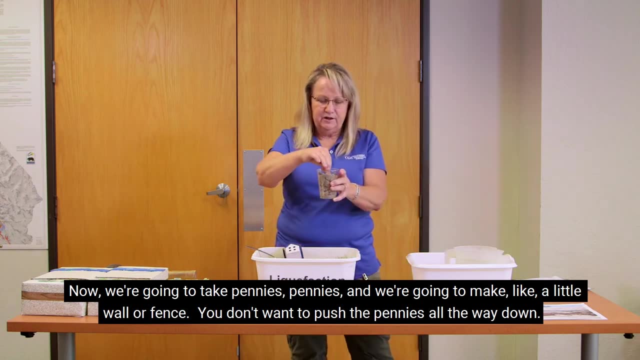 and we're not going to pack it down, but we're just going to make a smooth surface at the top. So there's spaces and voids and there's still water in there and we're going to take pennies, pennies and we're going to make like a little wall or fence. You don't want to. 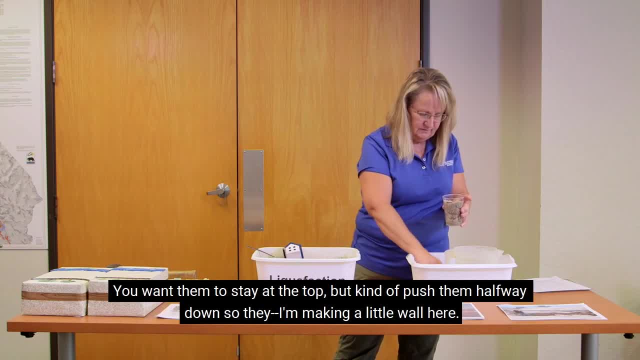 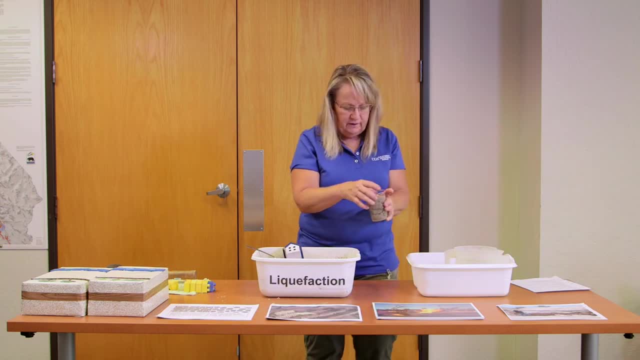 push the pennies all the way down. You want them to stay at the top, but kind of push them halfway down, So by making a little wall here and then I'm going to use my spoon again and I'm going to cause an earthquake.